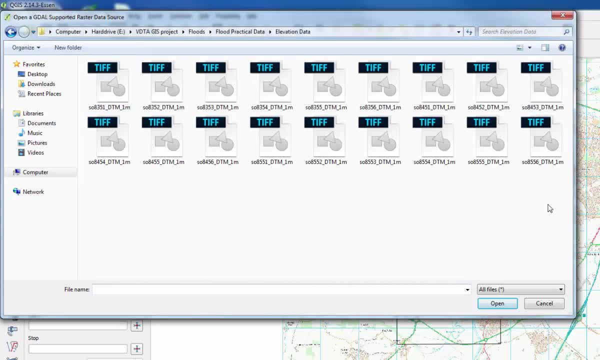 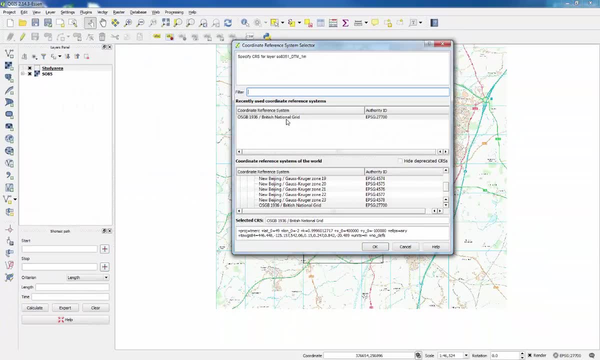 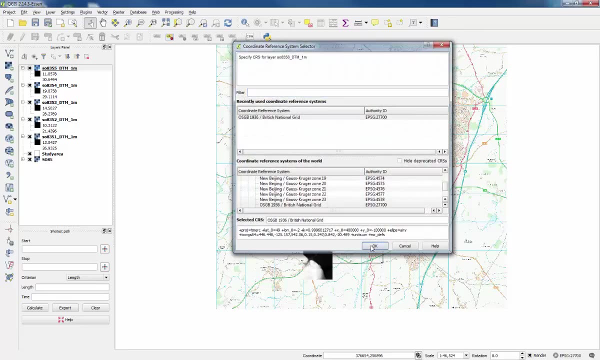 to the project folder, go to add elevation data here, highlight everything in this folder, click open. Then you need to confirm the coordinate reference system for each tile individually. so you've just got to press ok through all of those, which I'll speed up just a little bit Once you've done all of that. 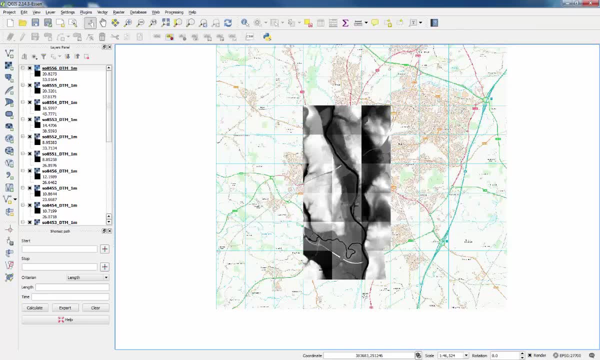 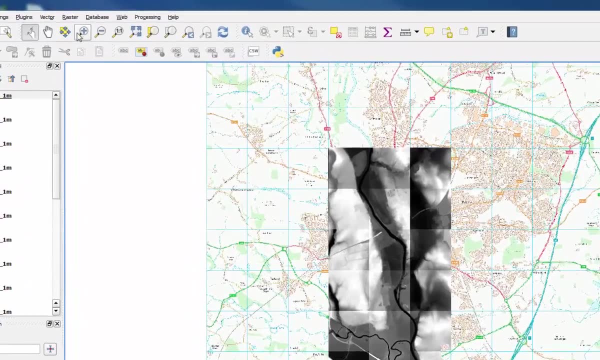 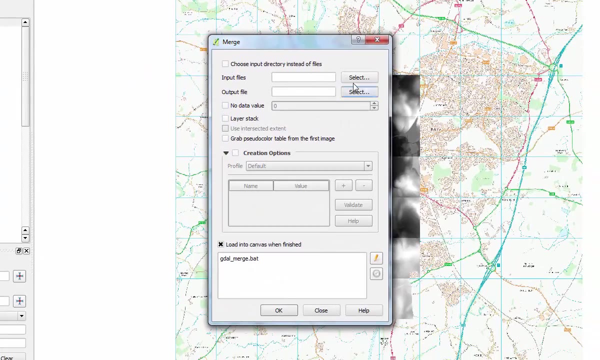 you'll have 18 individual elevation tiles on your map layout, So we can make this into one smooth, continuous layer by using the merge tool which you can find on the toolbar. Go to the raster tab, miscellaneous, and go to merge. The input files will just be all of the elevation data that we just opened. so highlight. 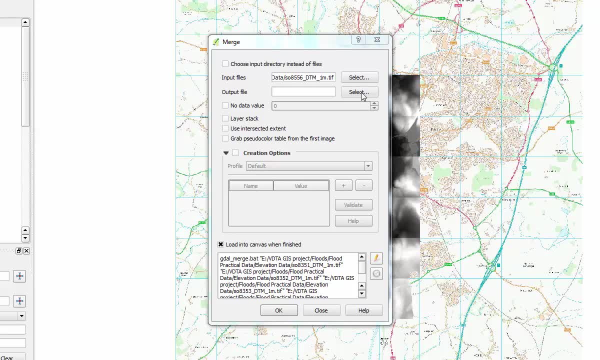 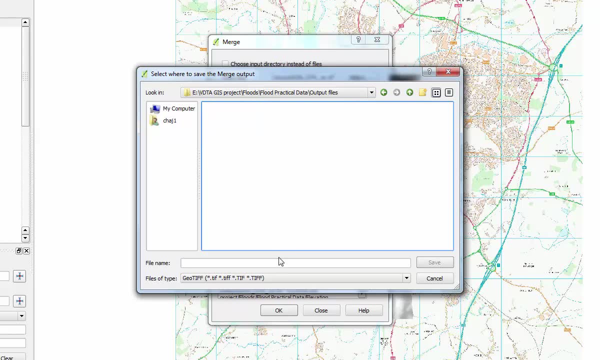 everything again. Click open and for the output file you just need to go to select and choose location to save the file. so it's going to be output files, just to keep everything tidy and give it a name, just something simple. Click save and then you. 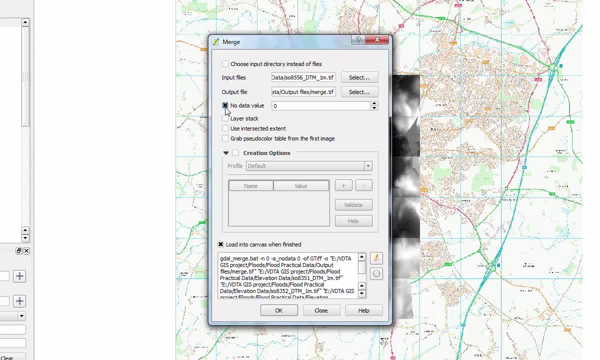 need to make sure you put a cross in the no data value box here. This means that any areas that have no data will be given the value 0, and then make sure there's a cross in the load into canvas when finished button Click. ok, wait for. 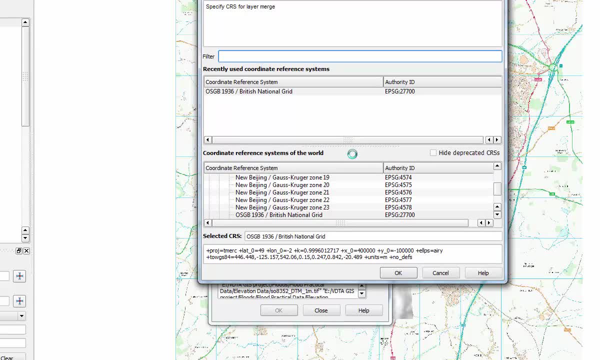 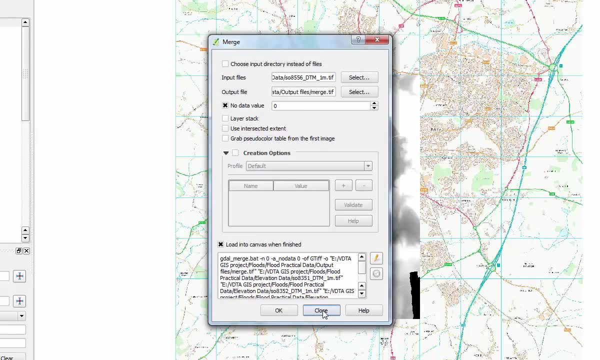 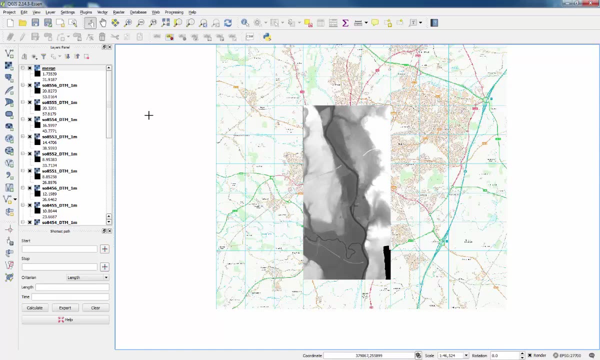 the tool to finish. Then, once it's completed, you have to confirm the coordinate reference system again. Click ok, ok, through the dialog boxes, close the merge window and you can see our mosaics raster elevation layer here, So you can tidy up the layers panel. 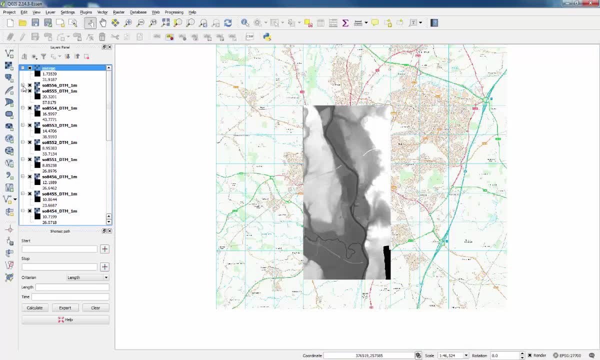 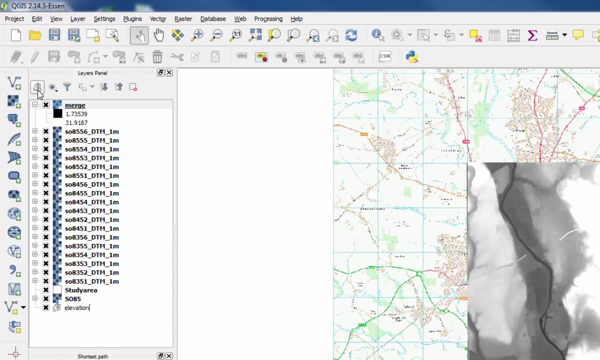 a little bit because there's a lot going on. So if we first collapse all of the original elevation data layers and then use the add group button to put a group at the bottom of the layers panel there, Let's call it something again, something simple, elevation, and then you can use click and shift to highlight them all. 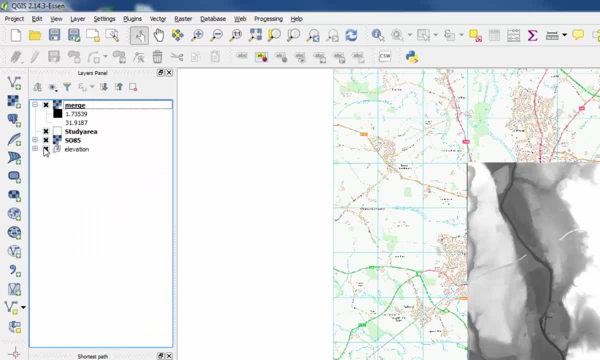 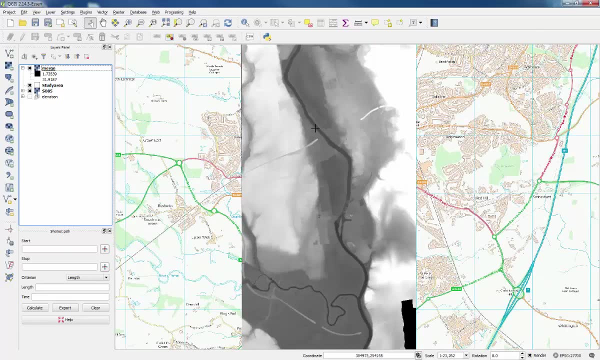 and then drag them into the new folder. You can collapse the folder and turn it off because we don't need it anymore and be left with the merged elevation layer here. So to make it look a bit more interesting, we can give it a 3d look. 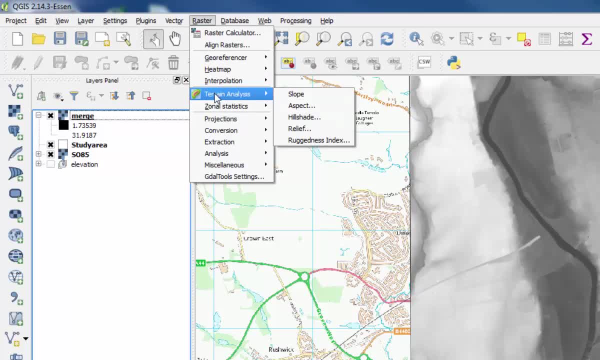 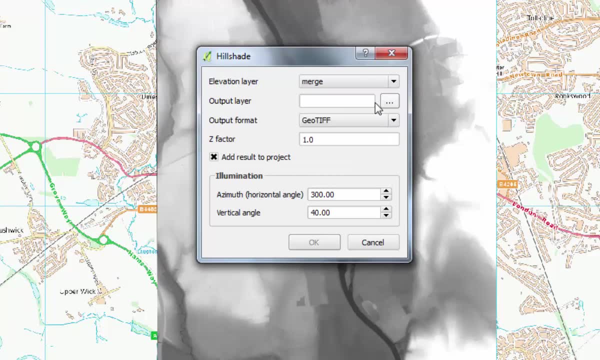 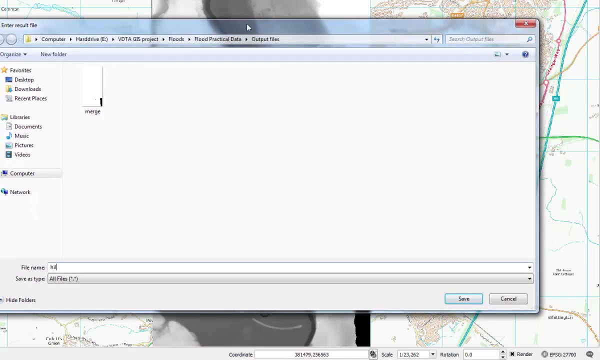 Again go to the raster tab. for this time go to terrain analysis and hill shade. The elevation layer needs to be changed to the merge layer, the one that we just created, and then the output layer. For this, again, just give it something simple. so this is going to be a hill shade, Click Save and then you don't need to. 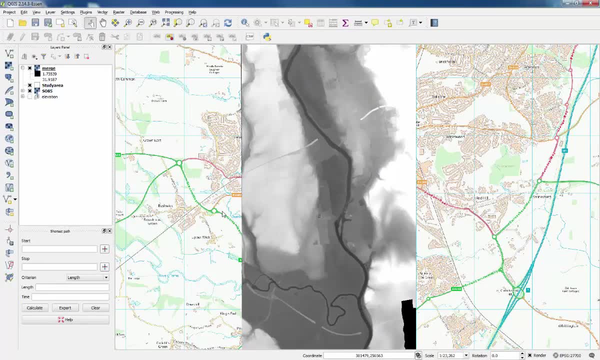 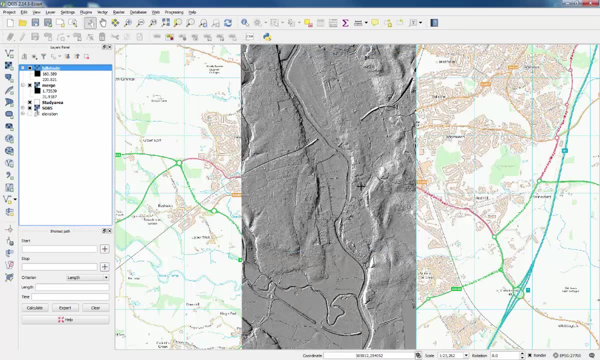 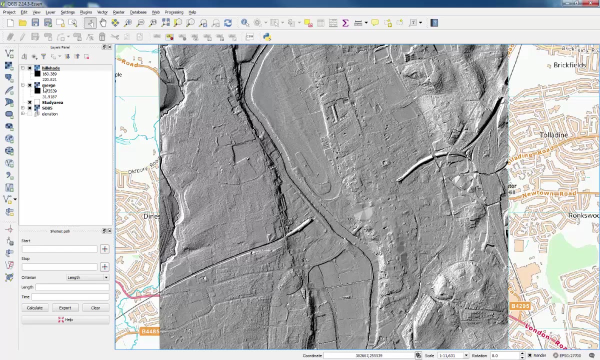 change anything else here. Click ok and wait for that tool to finish. Again ok on the British National Grid, and it brings up a grainy layer that looks like tinfoil really. So if you zoom in you can see some detail there, So we can make it look even better. if we just collapse those. Put the merged 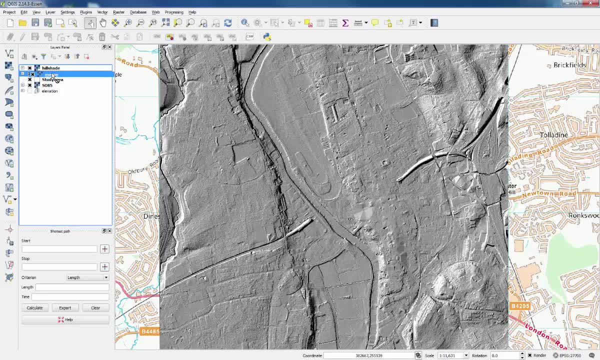 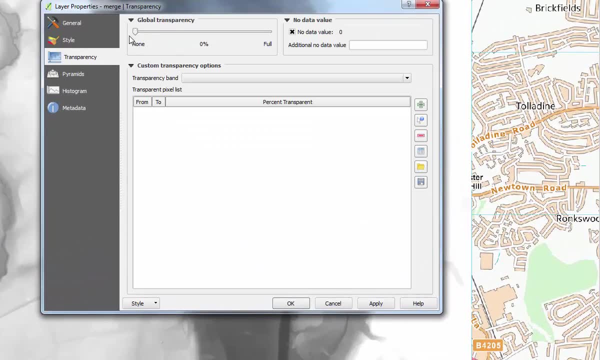 elevation layer above it on the layers panel and then double click to open the properties. again On the transparency tab, move the slider to about 40%. we're going to make it 40% transparent so we can see the hill shade layer beneath it. 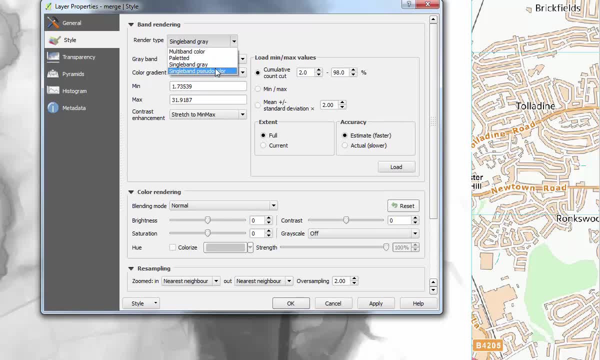 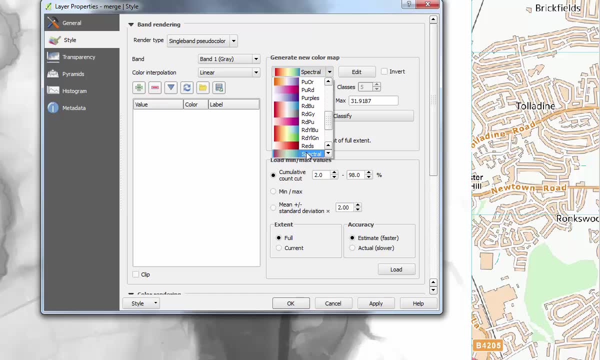 And then go to the style tab and change the render to single band pseudo color, Which gives us access to these color ramps. here You can choose anyone you like, but spectral works just fine. And then to change it from continuous, so just looking like the color ramp. you can give it equal intervals and choose the number of 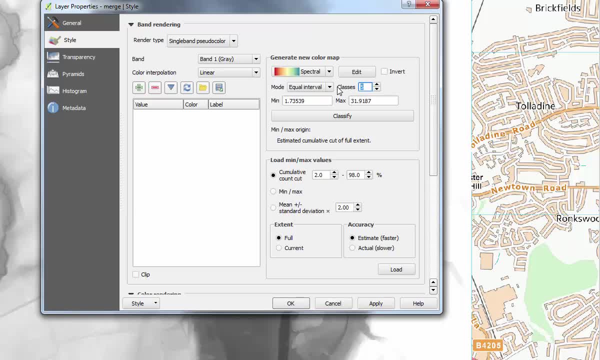 classes that the color ramp contains. So we'll go for 15 works and then click classify. So the values here are the elevation values at which the color will change. So you'll be able to tell from the color the exact elevation. So that's. 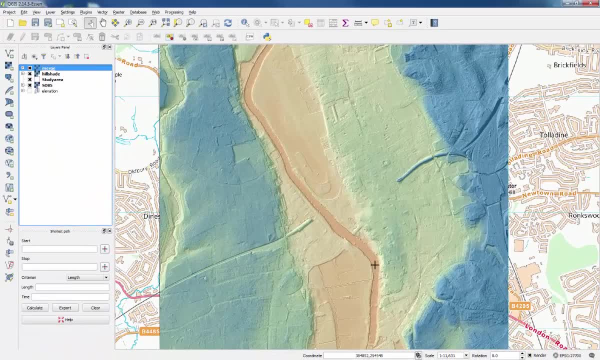 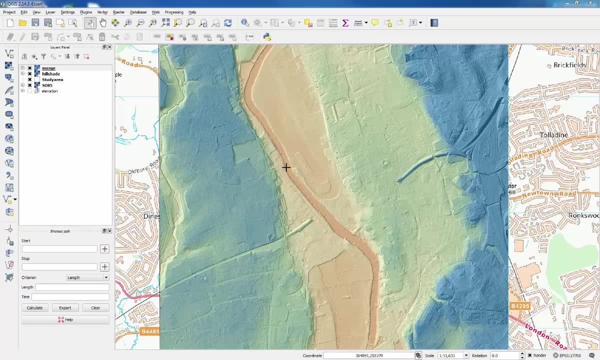 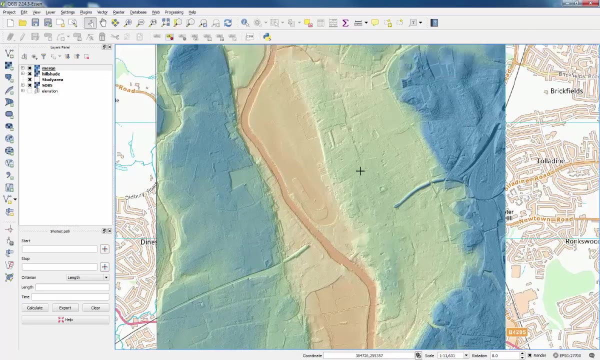 it. So click OK. Then that will apply the changes And you can see that the darker colors, the more red colors are lower elevation, and then the darker the blue, the higher the elevation. So the next step in the practical is to add the 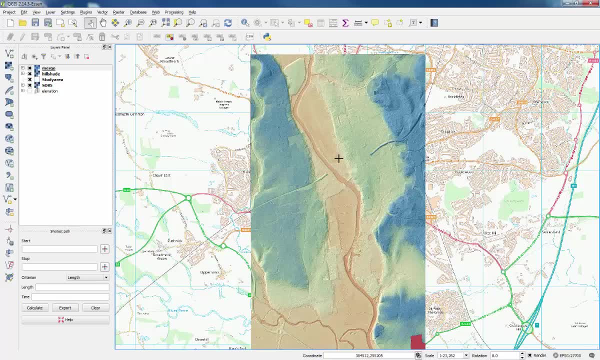 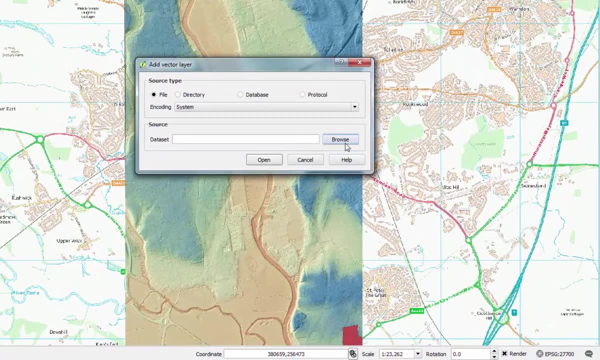 vector data from the ordnance survey So we can see the buildings, roads, the railways and the river. So if you go back to the add vector layer and then go to browse, Then ordnance survey vector data Open the subfolder and we just need to use the. 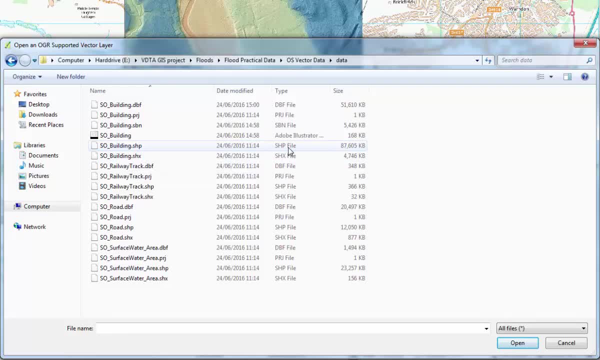 files that end in shp and have shp file under the type column. So you click each one and if you hold control then you'll be able to click all four of them at the same time. to save you coming back, Then just click open and open again and you'll. 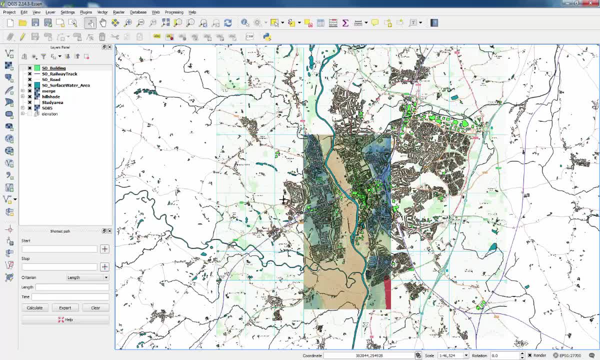 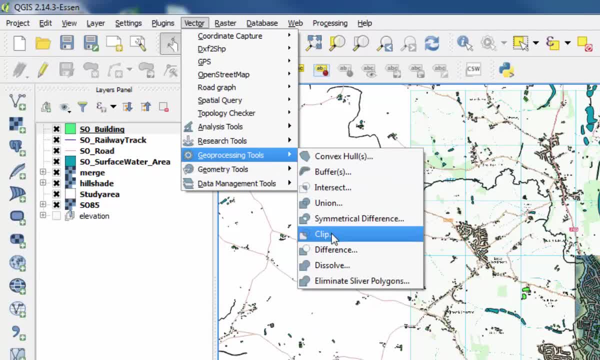 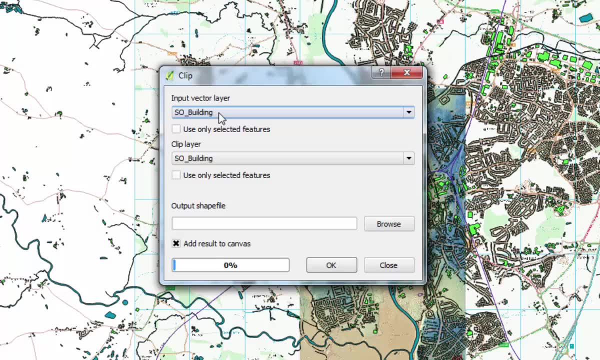 vector and then geoprocessing tools and find clip. Then the input vector layer is the layer which is being clipped. So in this case it's going to be the building layer and then the clip layer is the feature to which it's being clipped. 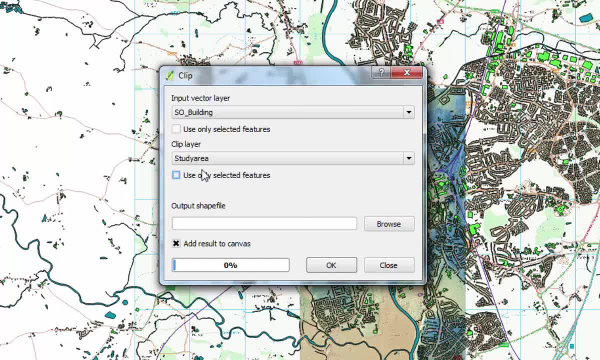 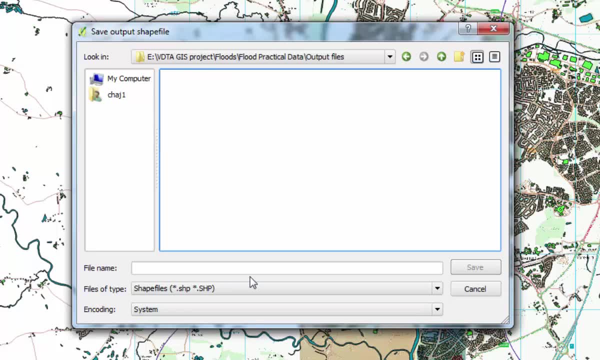 So that's going to be the study area, and you need to make sure to click on that each time because it will change. Click on browse to find where you're going to save the new shapefile. shapefile output files is fine, and then give it a name. something easy: buildings. 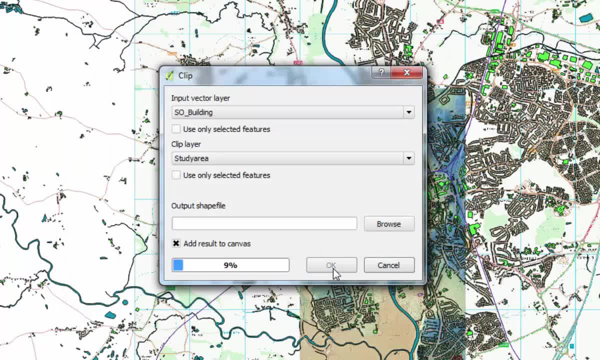 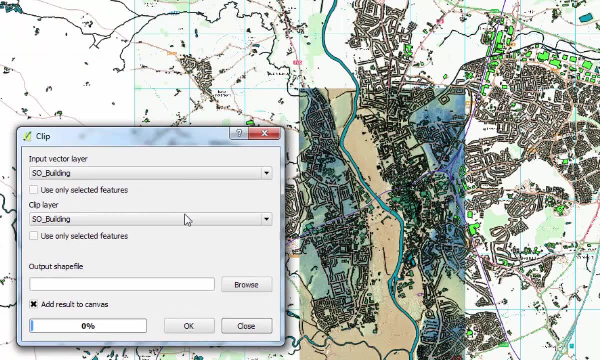 clip, click Save, then click OK. this one takes a little while, so I'll speed up the video here once that's finished. if you move the window, you'll be able to see that the buildings have taken on a different color inside the study area. so we don't need to close the clip window. you can just choose the next layer, which. 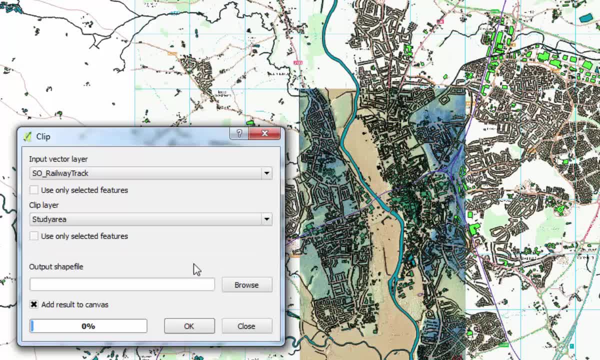 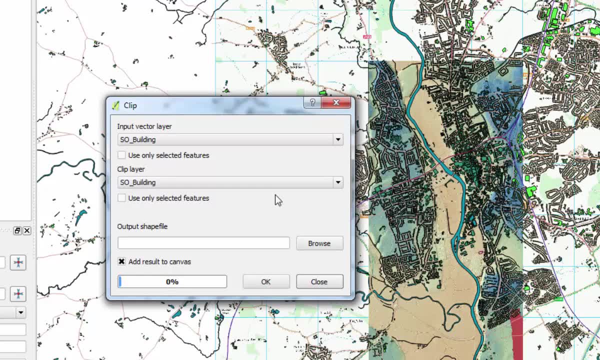 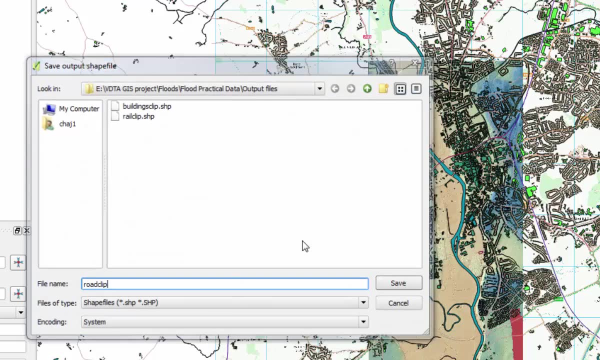 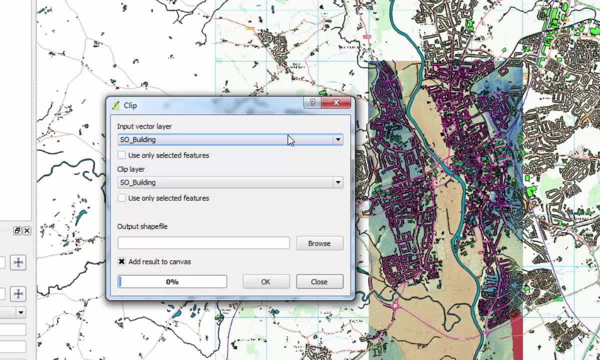 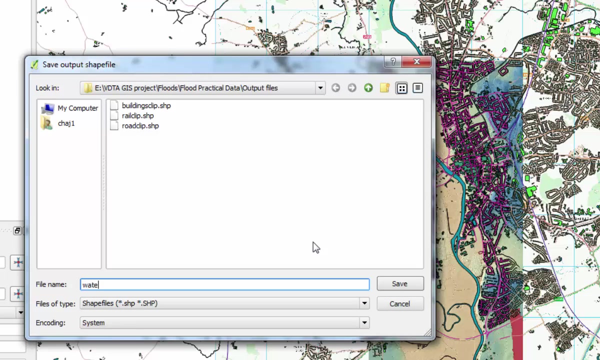 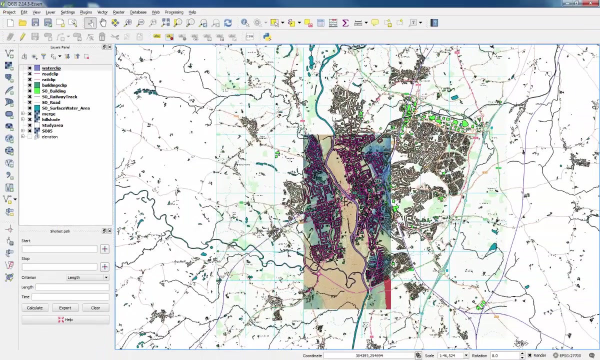 will be railway tracks. change the clip layer again to study area, then give it another name, click OK, and then we'll go through that again for the roads, okay. and and last time for surface water, change it to study area again. we'll call that water clip save and ok. then you can close that window. then what that lets us do is 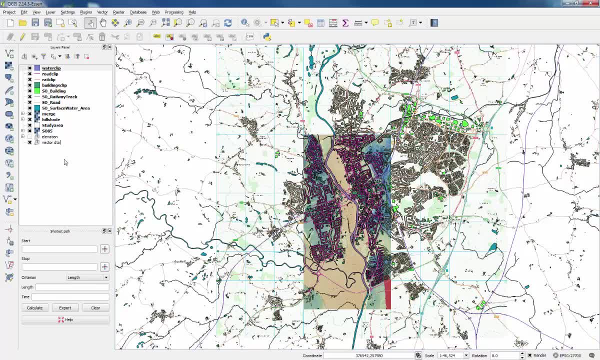 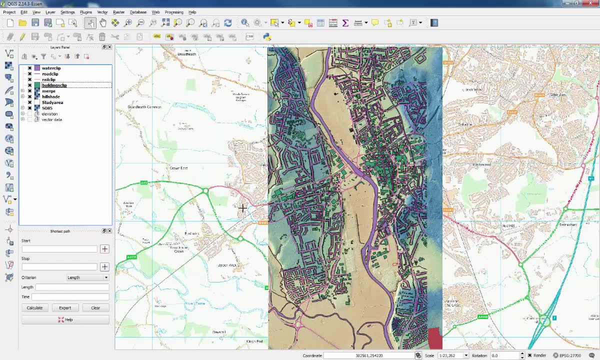 create another folder here. we'll call that one vector data. let's put all of the original vector layers into that folder, then collapse that and turn it off again. so we've just got the vector data in the study area. now you can change the colors of the data. 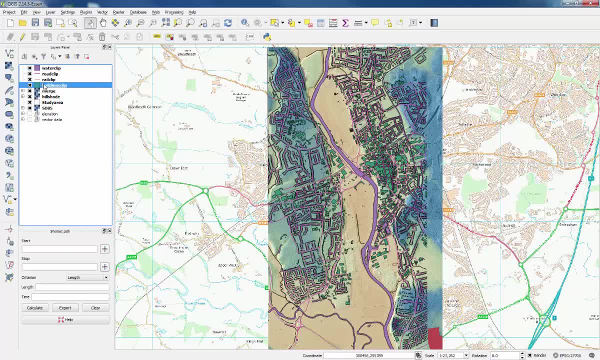 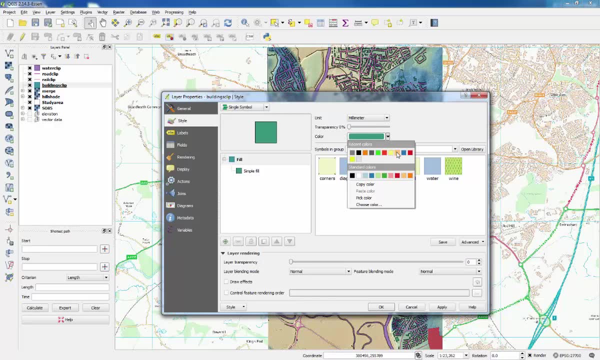 that are in this study area now by double-clicking on its name in the layer panel and go to style again. so we're on buildings. so with the ordnance survey, they're usually an orange color, so we'll choose this one and click OK- railways. 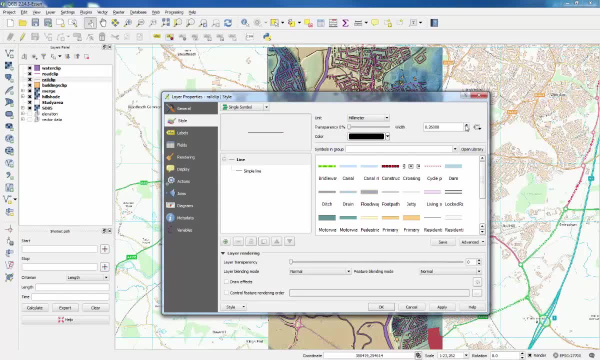 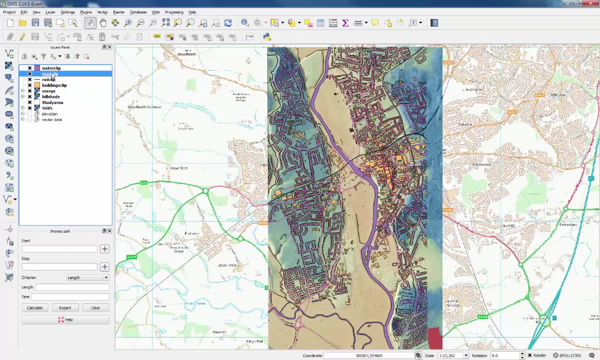 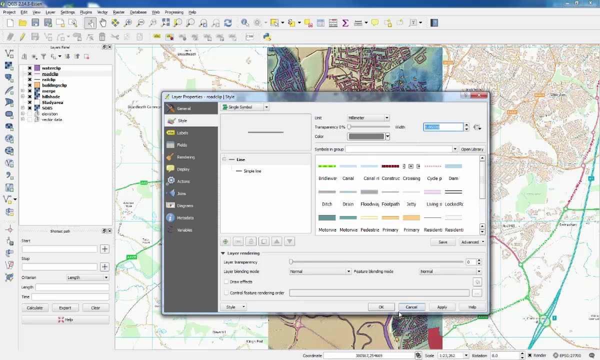 are usually quite thin black line, so you can change the width of the line using the up and down arrows here or entering some value into that box. and we'll do the same with the roads. we'll make them a kind of realistic gray color, make those a bit thicker so they stand out a bit more. and then the water. 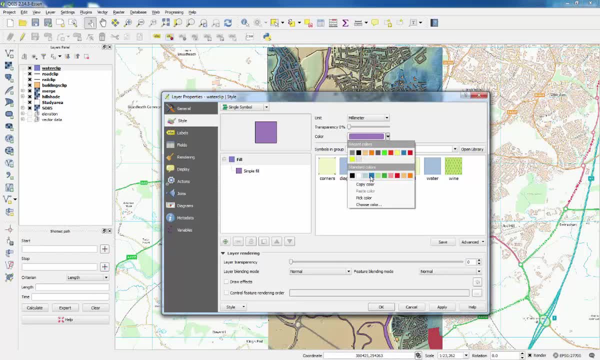 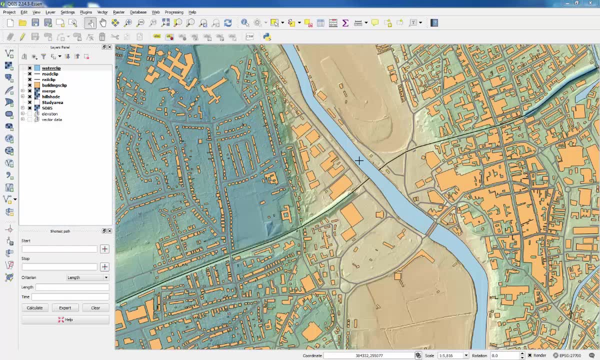 will change that from purple, we'll make that blue and ok. so if you zoom in here, you'll see that the water actually goes over the railway, which we can change just by rearranging them in the layers panel. put in water at the bottom. it's a bit more realistic now. then the next step is to add the flood risk data. 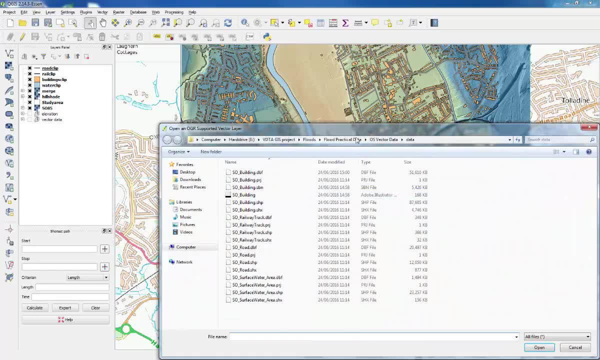 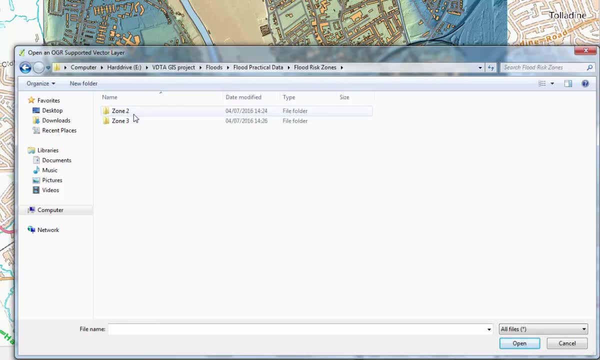 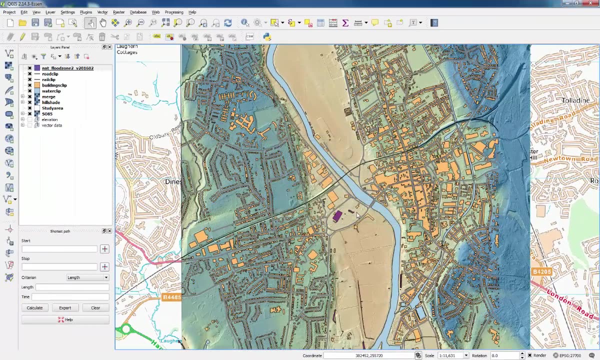 so it's vector data again. go back to browse and back to the project folder. then find the folder that says flood risk zones. open this one and you get the option of zone two or three. we just go with two first and then find the shape file, click open and open again, and it doesn't seem to do anything. but if we 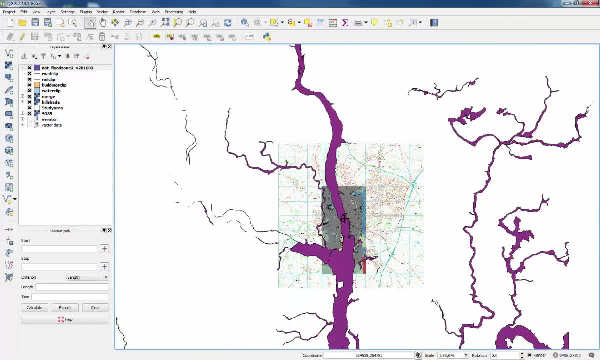 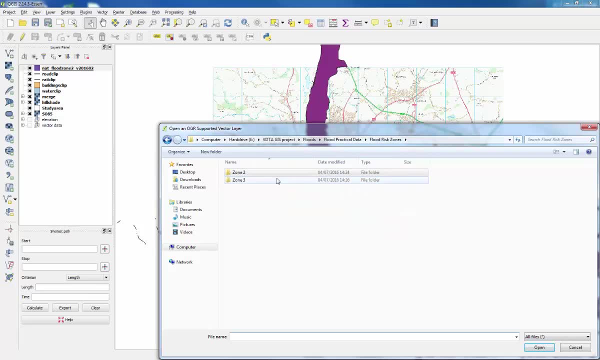 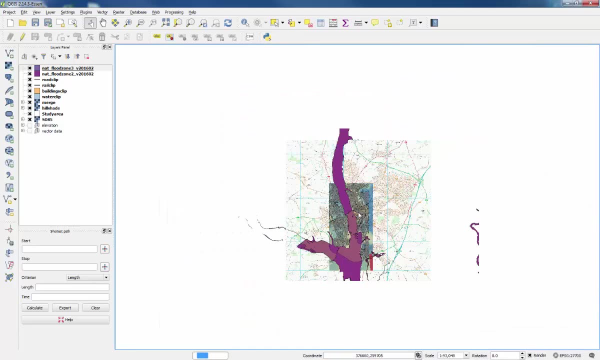 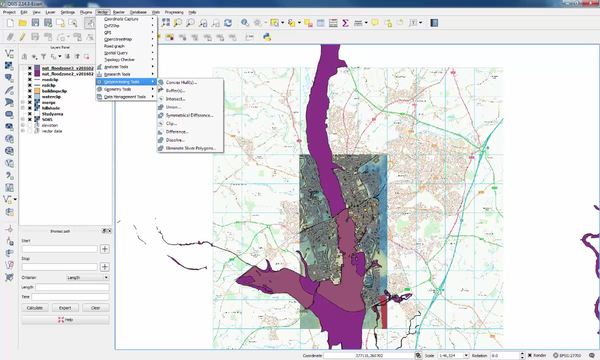 zoom out, then we can see it is part of a bigger layer. so we'll clip that afterwards. we'll just add the second layer, flood risk zones, and zone three shape file. now click open and again that lays over the top of zone two. so if we go back to vector and geo processing tools, go to clip, change the. 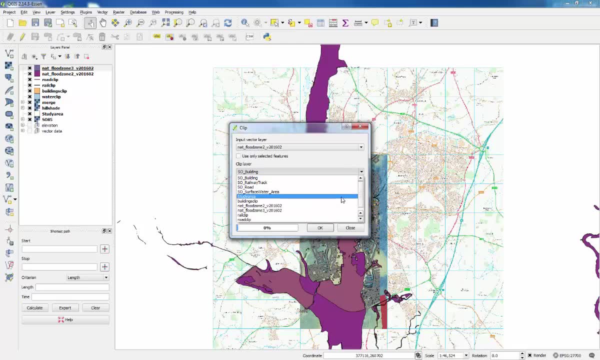 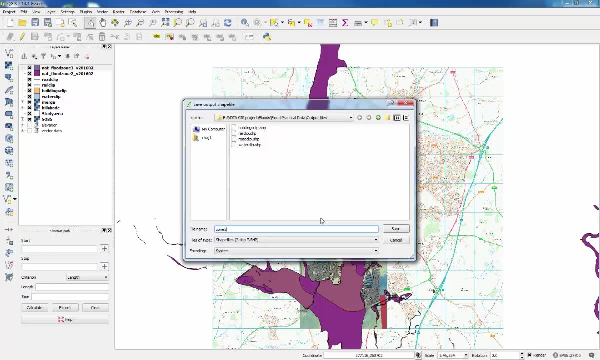 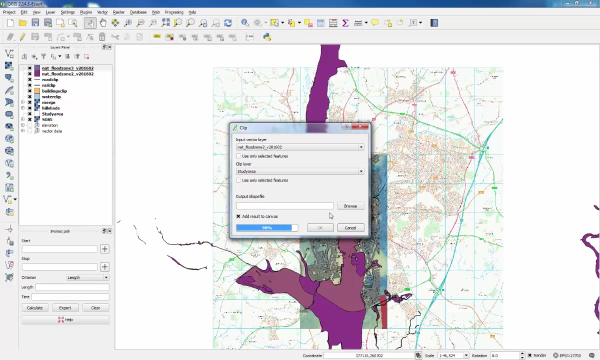 input vector layer to zone two. we're clipping it to the study area. we'll go to browse. we're still in the actual study area. we're still in the actual study area output files folder. we'll put in zone two, clip and then okay, and then we'll. 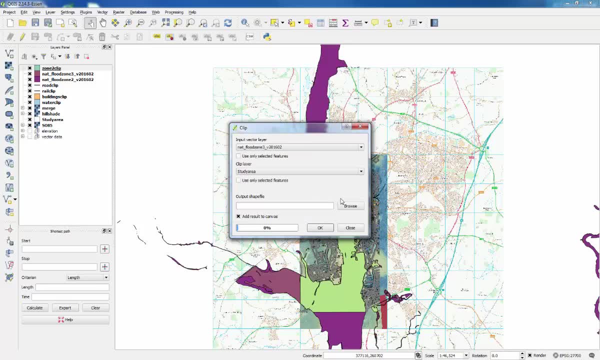 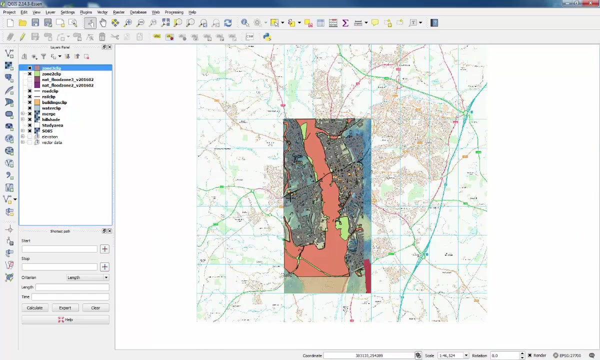 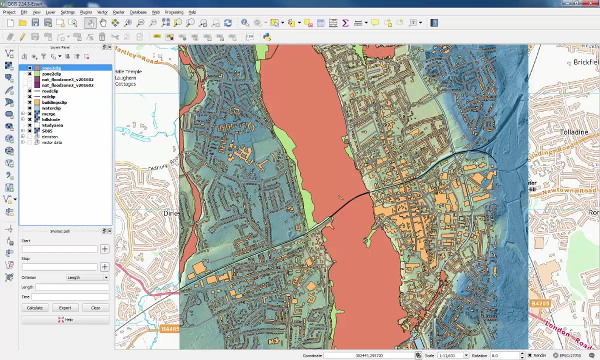 find the same three layer and then we'll find the study area again, zone three clip. save that and okay and click close to close the clip window and then we can switch off the original flood zone layers. so that leaves us with the layers. they're quite opaque so we can change those and see which buildings are going to be. 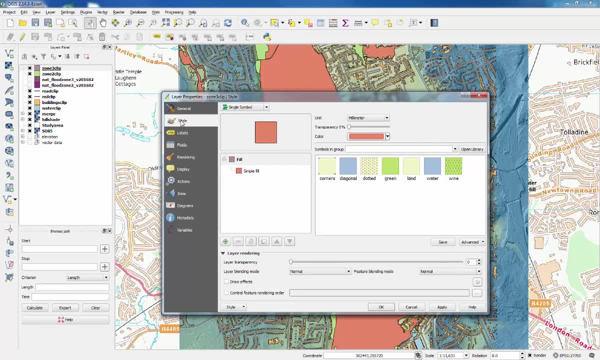 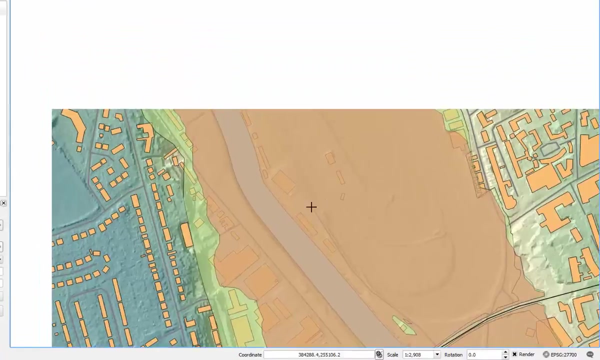 affected by the flooding because it's vector data. the transparency is under the style tab, so just move the slider to about 50% and okay. then do the same for zone two and click okay, and you can see which buildings should be affected by different levels of flood. then the final feature that we could add was the: 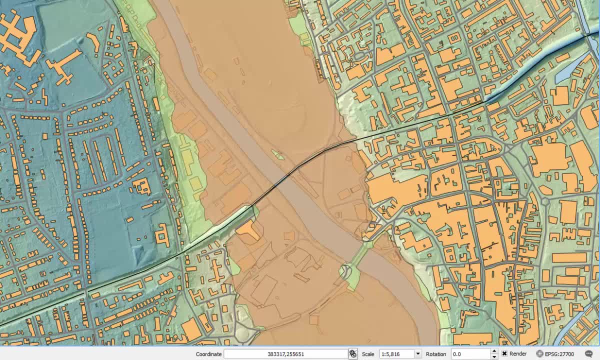 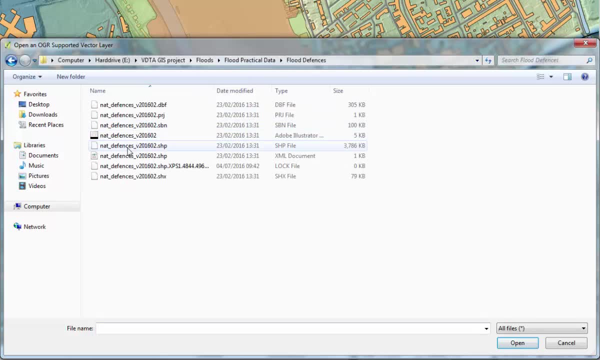 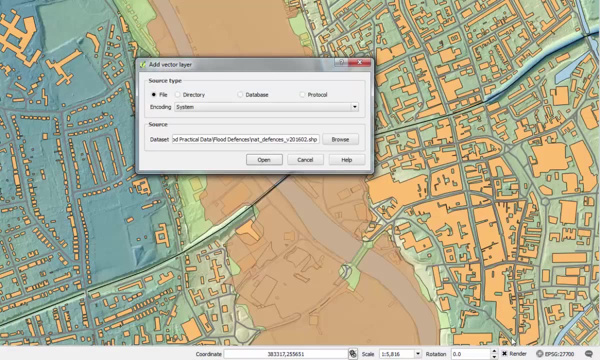 flood defences. thats vector data again. so back to the project folder flood defences. find the Nacional defences shape file with the SHP file and a flood defences type there. open that one and it doesn't seem to do much. we'll put it above the. 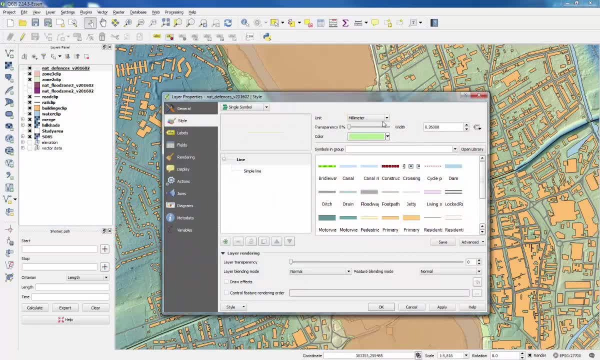 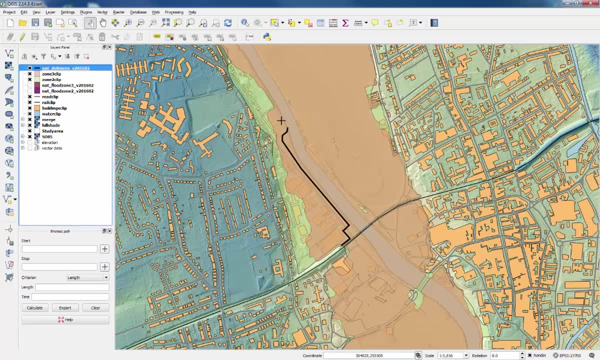 flood zones, and then we'll change the color so it stands out a bit more. make it black and change the thickness, and there we can see the flood defenses along Hilton Road. so that brings us to the end of the practical. don't forget to have a go at the questions on the handout. have a go at the quiz on. 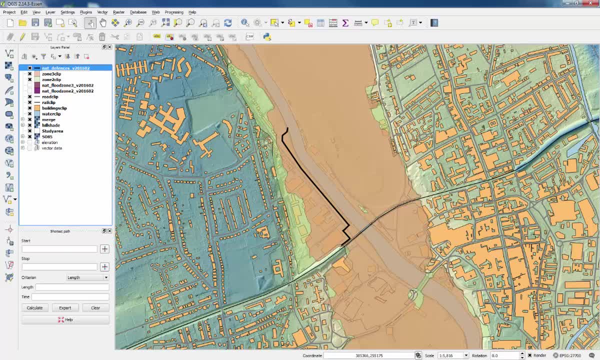 blackboard, if you can, and have a look at some of the other practicals as well. 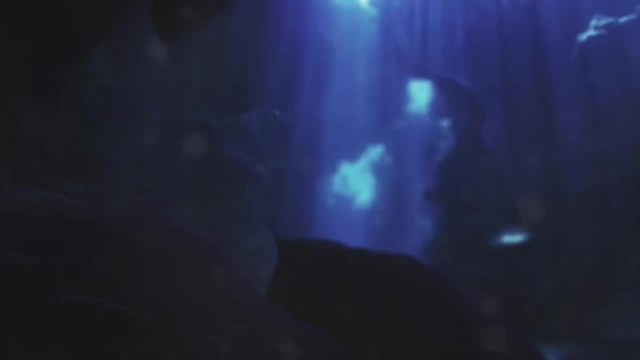 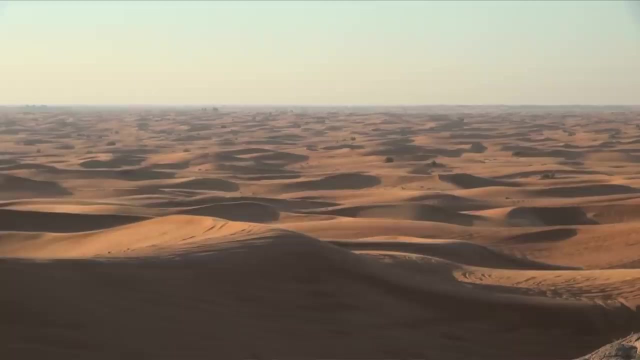 Imagine a world so warm that the ocean feels like a hot tub. Huge volcanic eruptions have pumped the air full of globe-warming carbon dioxide And with the continents locked together from pole to pole in the supercontinent of Pangea, the world is hot, flat and very. 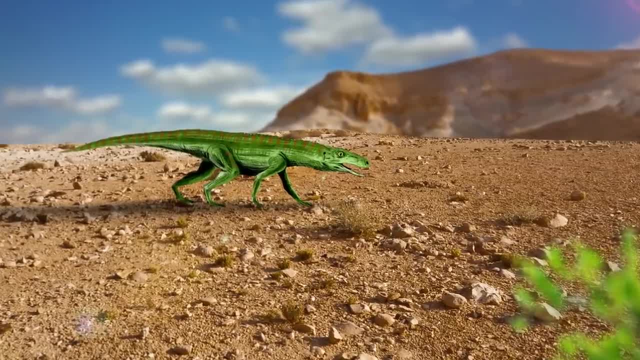 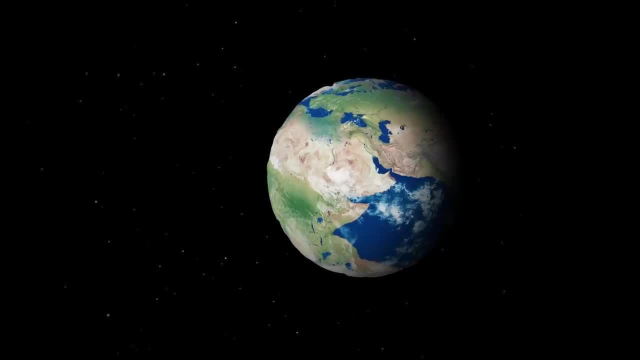 very dry Early reptiles and mammal ancestors thrive in this sweltering land, dominating a landscape that's still struggling to recover from their Permian extinction. This is Earth 250 million years ago, at the beginning of the Triassic period, But then starting around 234 million.